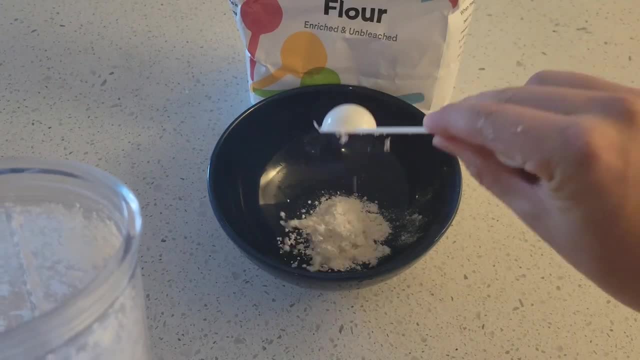 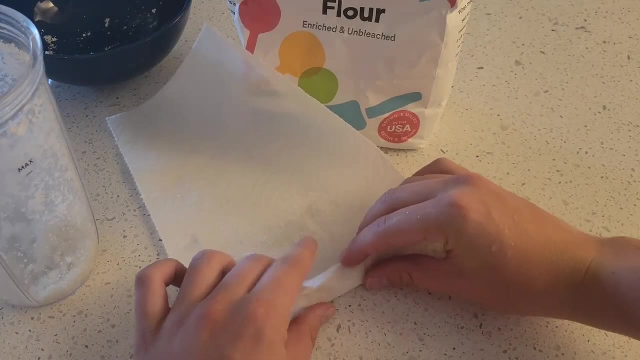 I decided to use a blender because it worked better. Then place a bit of flour into a bowl, Add a few scoops of crushed eggshell and a small amount of water, mush it up into a paste and shape it. Then roll it up and place it on the counter to dry for a few days. 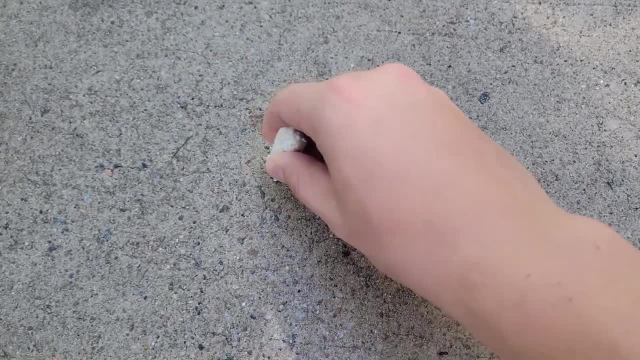 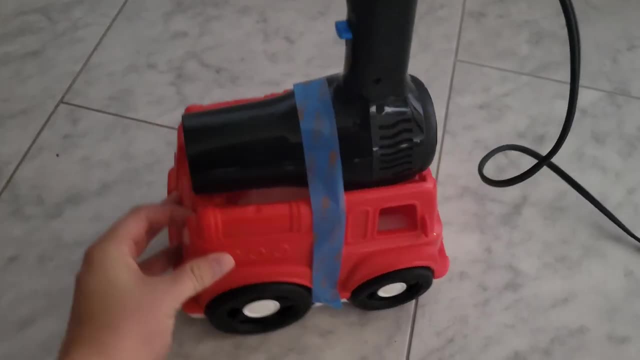 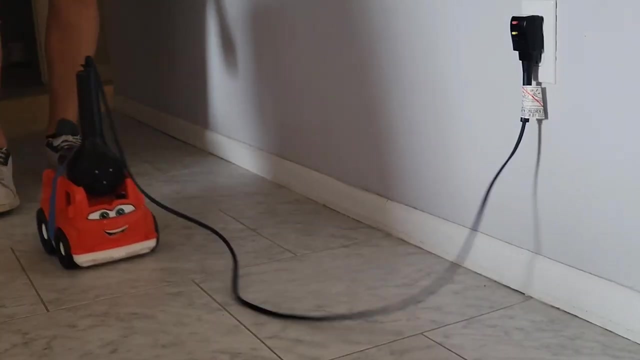 After waiting, you can take it out of the paper towel and it works like chalk. The rocket propellers use Newton's third law to move forward. In this example, air is forced out the back, meaning the card experiences an equal and opposite force that propels it forward. You've seen all three videos now. 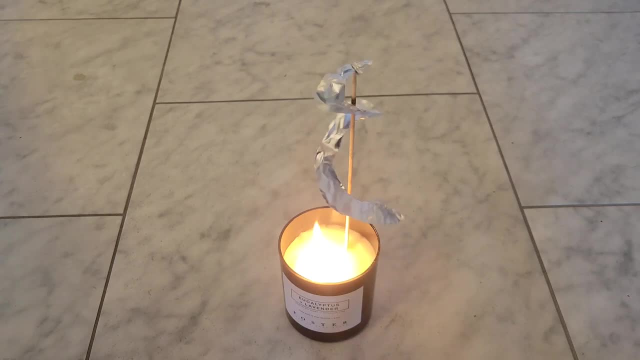 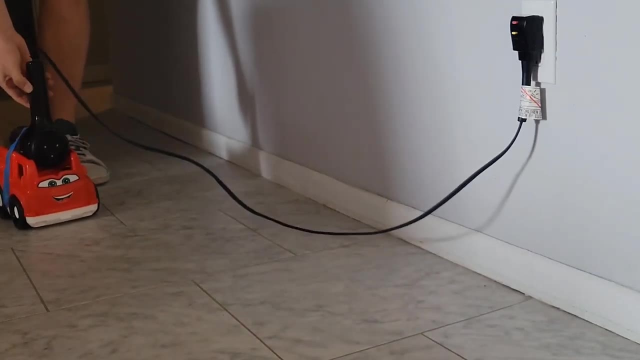 pause to vote in the comments, which one you thought was fake? The heat from the candle does actually spin the aluminum foil and, yes, this is a real recipe for creating chocolate. That means this one's fake. The hair dryer is not nearly strong enough to propel the car forward. 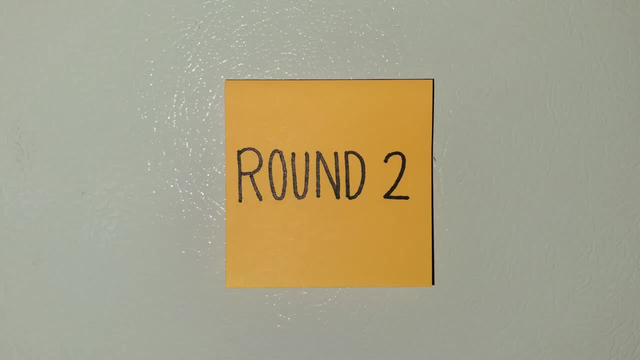 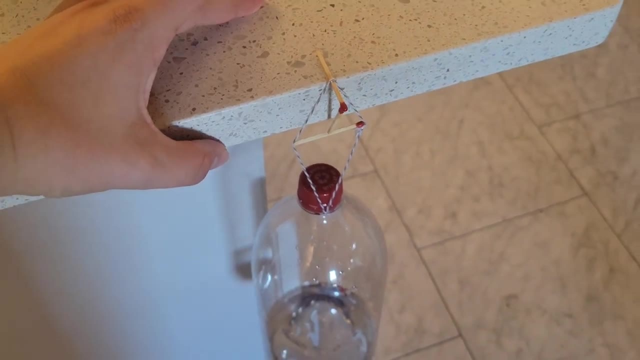 and the whole thing was put in reverse. Hopefully you got that one right, but if not, it's time for round two. If you place matches and string in a configuration like this, you can release your finger and it will still hold up a pretty heavy bottle- no glue necessary. 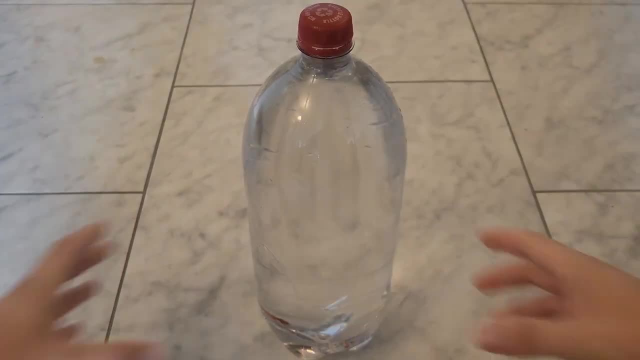 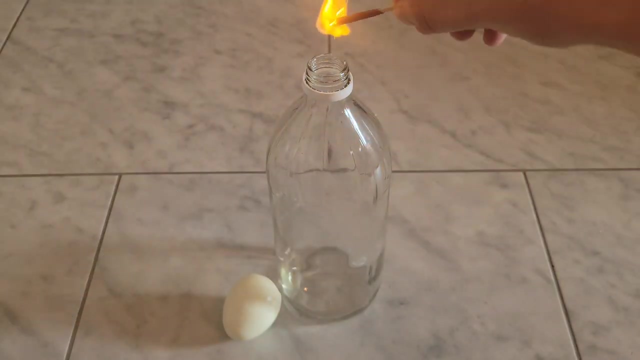 If you cut the tips of matches and put them in a 2 liter bottle full of water, you can squeeze the bottle and then the match tips will rise. If you light a match, drop it in a glass bottle and then balance an egg on top of the bottle, 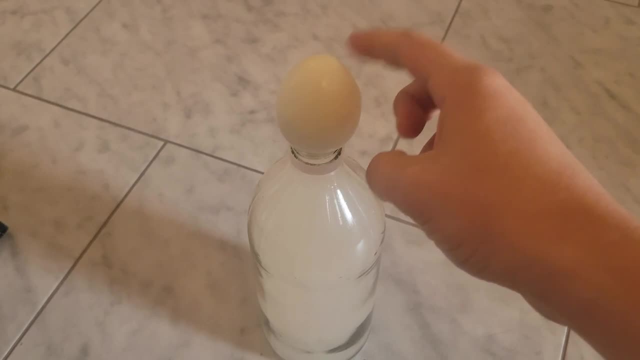 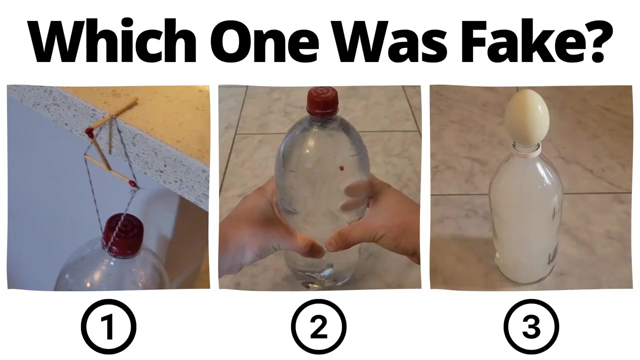 After waiting a few moments, you can successfully pick up the bottle with the egg. You've seen all three videos. now pause to vote in the comments which one you thought was fake. When the match goes out in the air, inside the container cools. 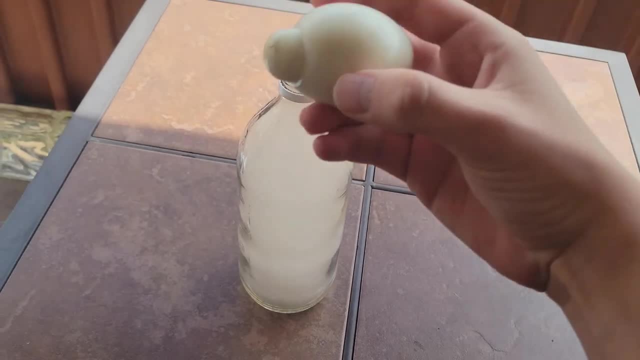 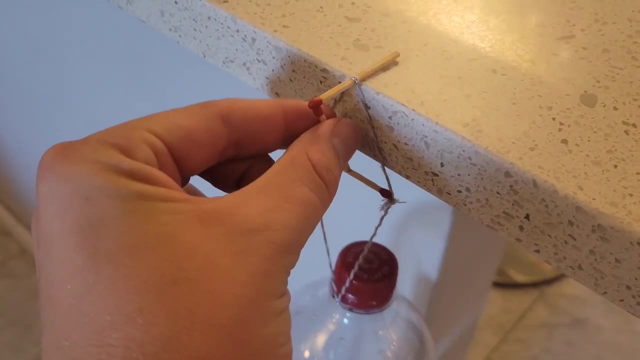 a partial vacuum is created that tries to suck the egg in. This egg was too large to get sucked in, but the suction was strong enough to lift the entire bottle. If you thought this balancing video was fake, well then you'd be wrong. That means this video is fake. The original video was in. 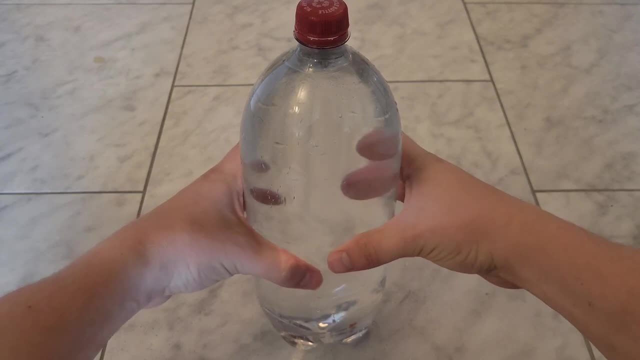 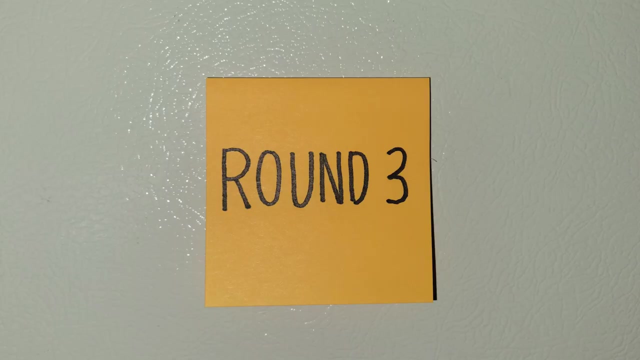 reverse. Match tips normally float in water, so squeezing the bottle compresses them, making their density slightly higher, just enough that they will now begin to sink. Next up, it's time for round three. If you place hand sanitizer on a plate and add Himalayan salt, 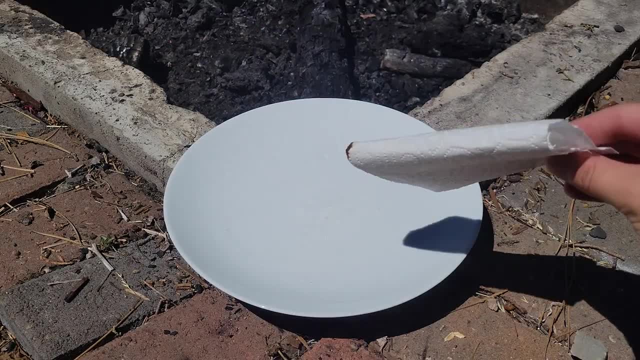 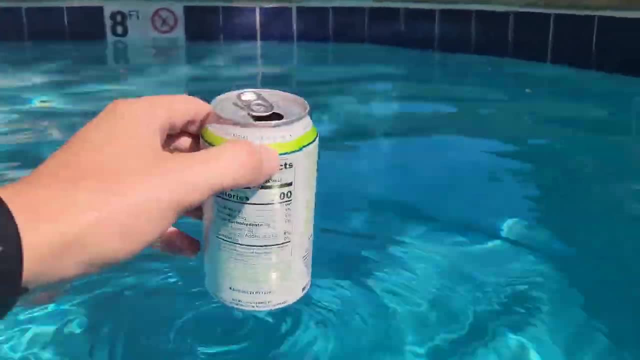 the reaction is dangerous if it comes into contact with a paper towel and the paper towel will catch on fire. An empty aluminum can has a hard time balancing on the surface of water without falling over, but if you let the air pocket underneath the can escape.